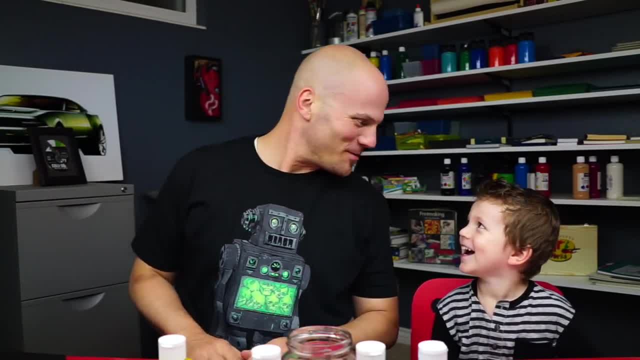 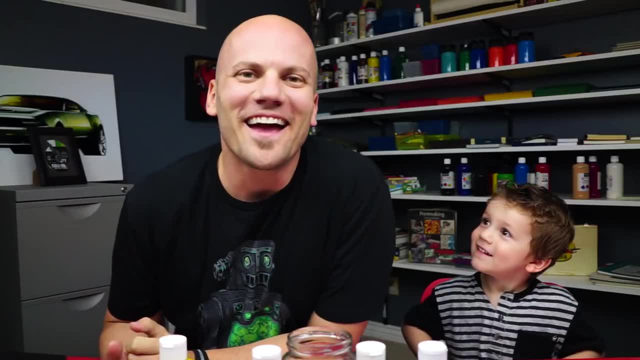 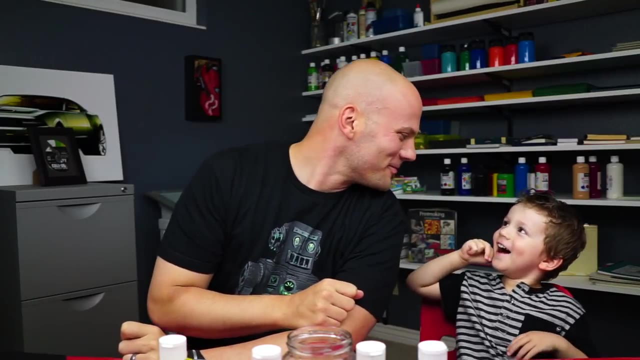 You ready? Yeah, Okay, You ready to paint? Yeah, Yeah, Okay, look at the art friends. Can you see them? Yeah, Yeah, Hey, art friends, I got my special little guest with me. What's your name? Um, No, what's your name? Austin, Austin, And you're two years old? huh, Yeah, Yes. 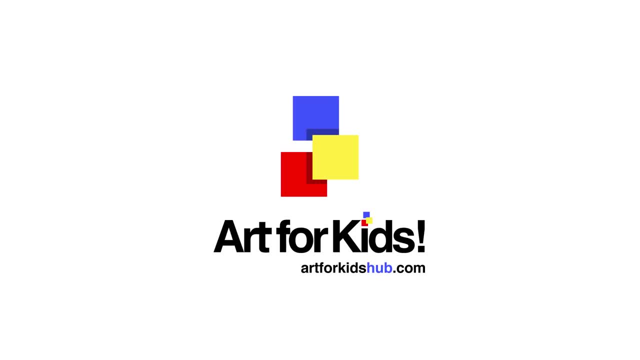 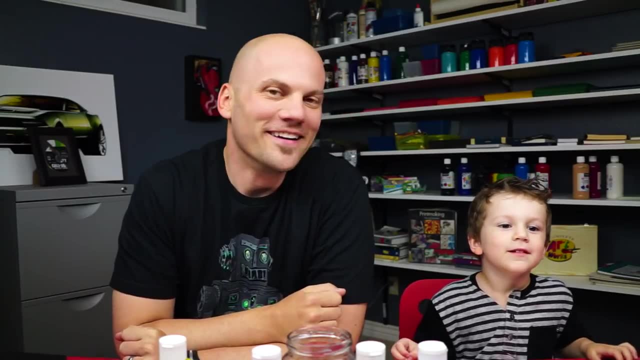 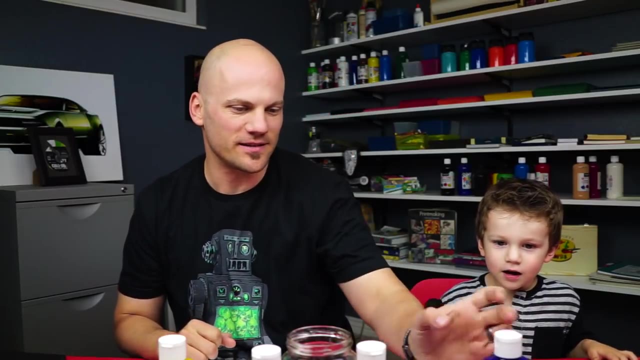 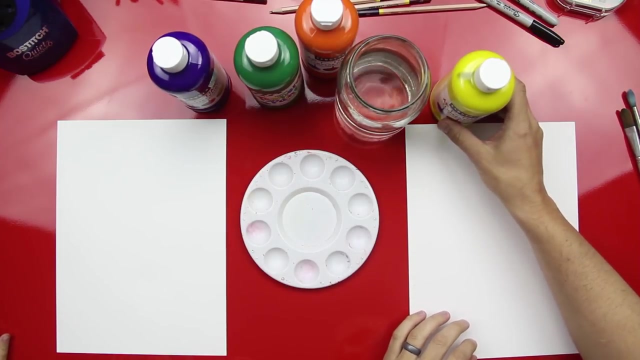 Yes, All right, Austin, what are we going to paint today? Do you remember Cactus? Yes, we're going to paint a cactus. So we got all our paints. huh Yeah, What colors do we have? What color is this? Purple, Purple. What color is that? Green, Green? What color is this? Orange? Yes, Yellow, Yellow. And we got our paint tray. We got some special paper. It's. 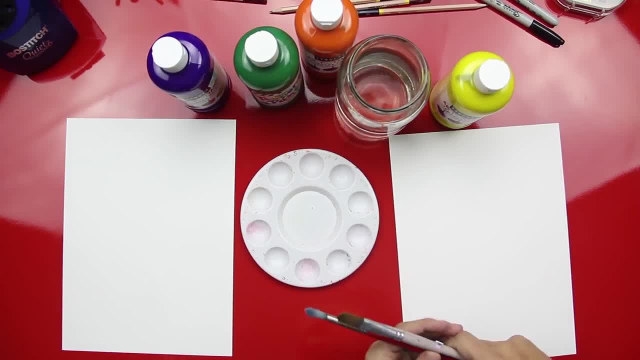 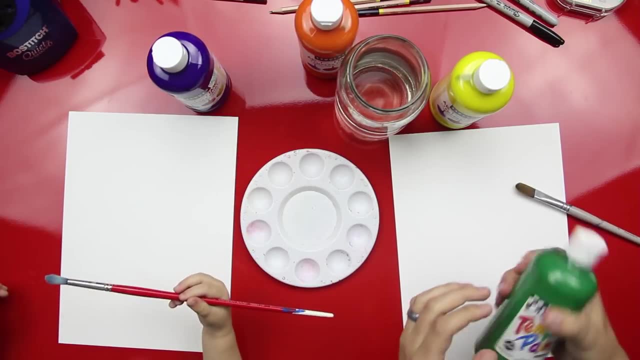 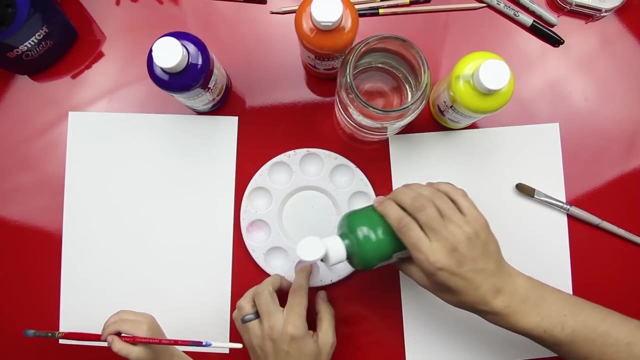 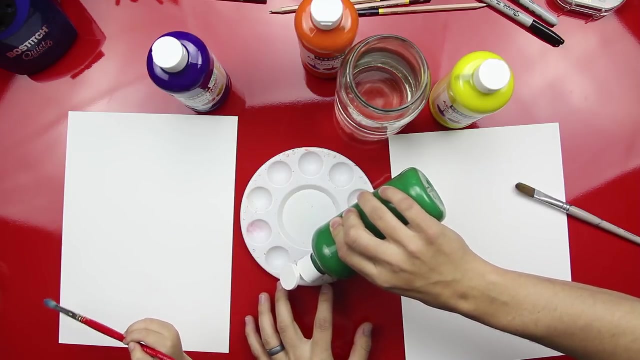 a little thicker than computer paper. And then we also got our paint brushes. Yeah, You ready? Yeah, Okay, you want that one. Yeah, Dad will have this one. We're going to start with green And we're painting cactuses because it's summer and also because we live in a desert area, So we see cactuses once in a while when we go more south, But we have cactuses, huh, Uh-huh. So we got a lot of green. You ready, dude? Yeah, All right. 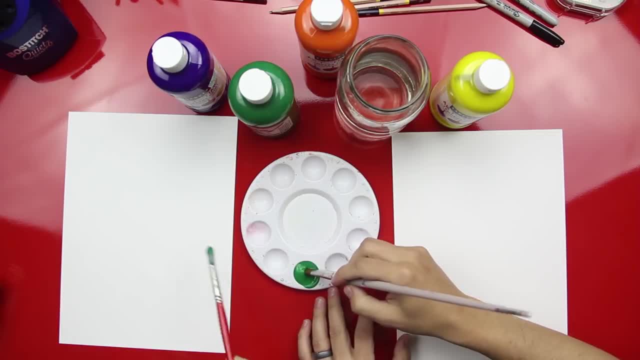 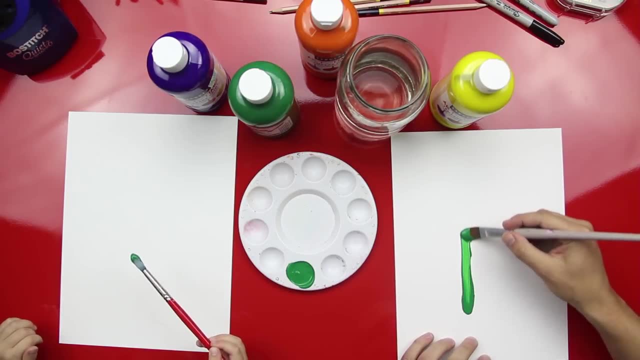 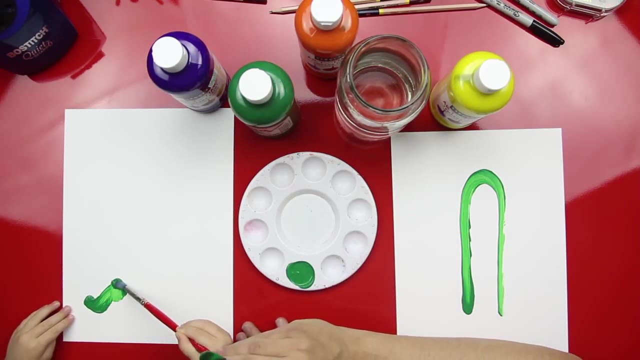 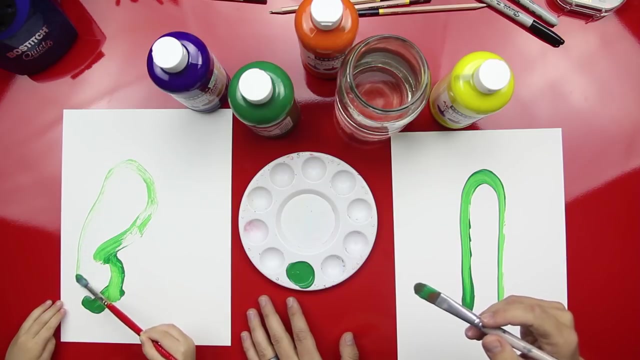 guys. Get some green on your paintbrush- Good job, Okay, watch this. Austin Watch dad. Okay, We're going to do a big Watch dad. We're going to do a big U like that. Can you do that? Yeah, Start in the middle, Yeah, And then go up, Go up here, Go up here And then down- Good job, All right. get a little more paint, Okay, And then we're going to fill it in. 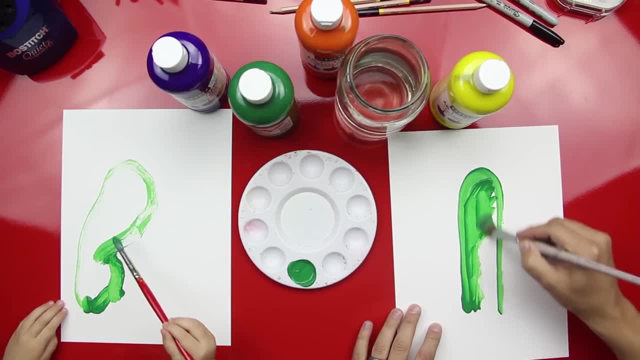 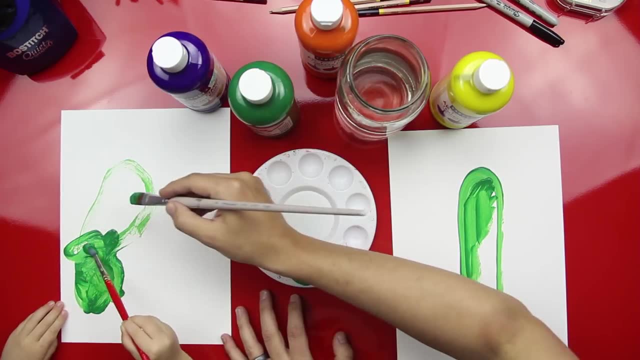 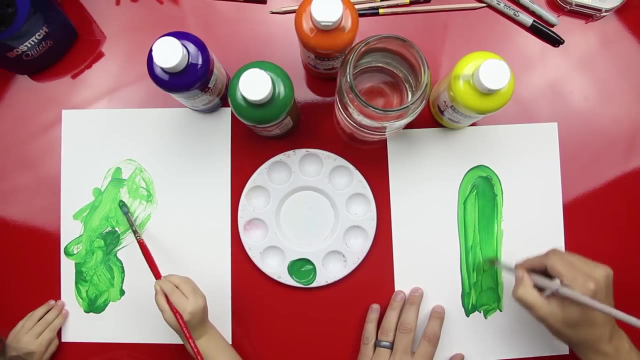 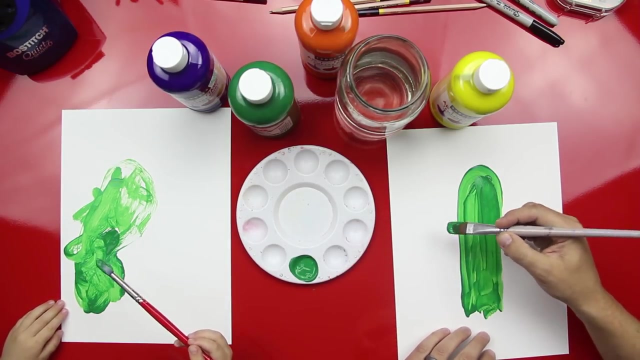 Can you fill it? Color in your cactus, Color in the middle. Yep, Yes, Good job. And then color, Paint up here too, In there, Inside. Got it? Okay, All right, We're going to do one more. Watch this, Watch this, Austin. Okay, Now we're going to make a four, Make a four. 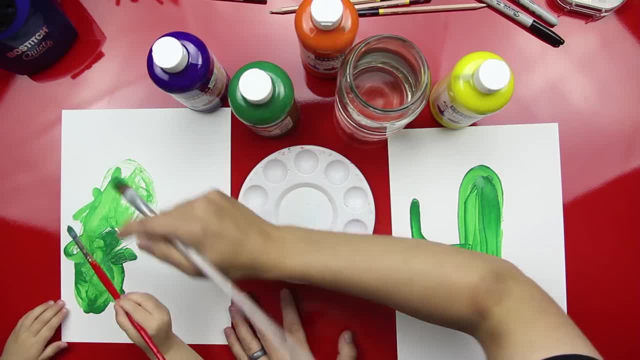 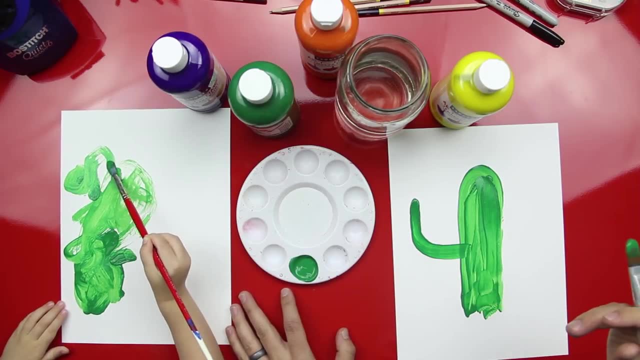 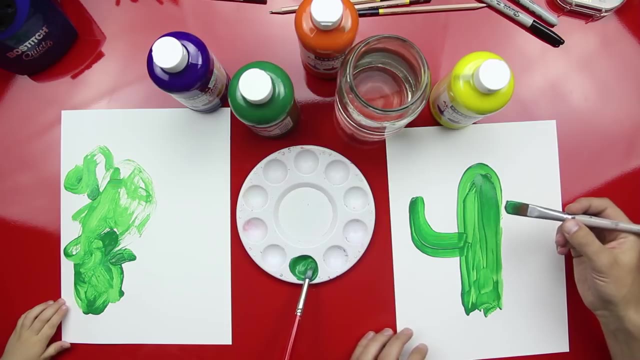 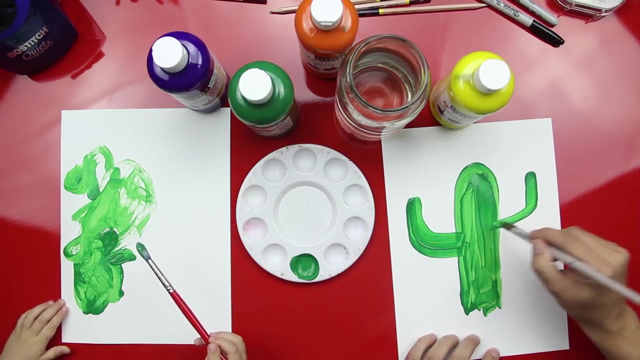 Do you want me to do that? Yeah, Right here, Do it up here And then go up. Okay, Yeah, that works too. Good job. Okay, Now watch, I'm going to do another four right next to it, But watch this, We're going to do another four on the other side. Okay, You're watching me. Okay, We're going to do another four over here. We go down and then in. Can you do that? 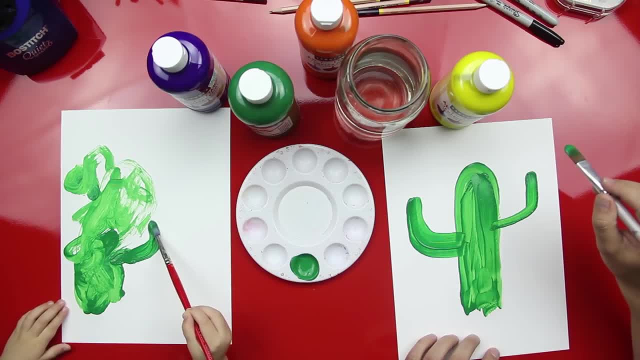 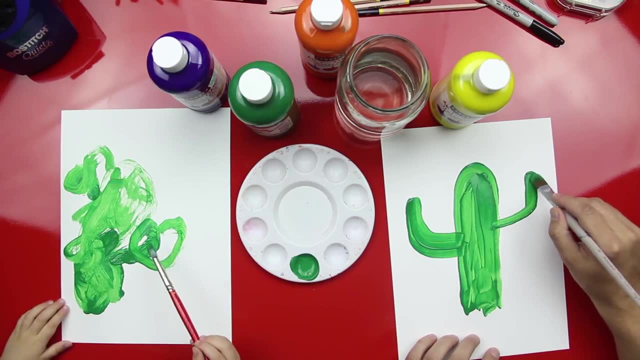 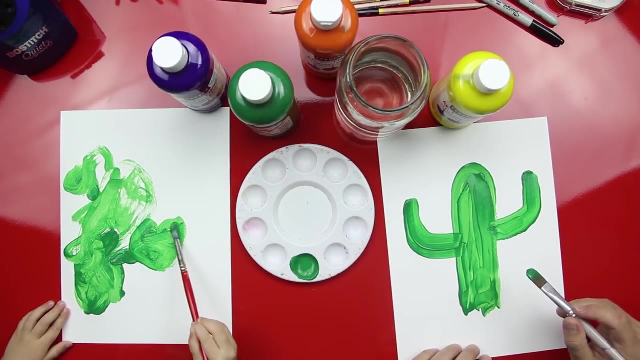 Yeah, We're going to go up. Good job. Oh, a little curly, Good, Okay. and then Dad's going to do one more four right next to it. You see that That is perfect. Austin Triangle, Triangle, Maybe. All right, okay, now we're going. 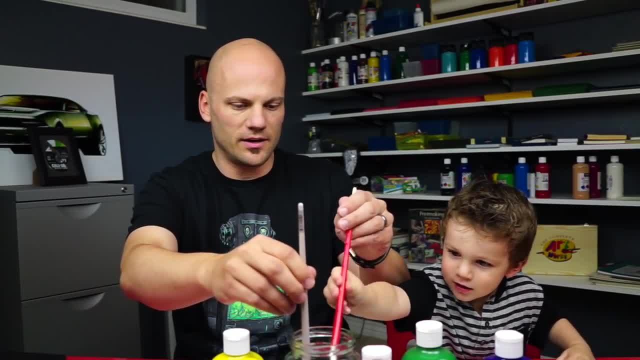 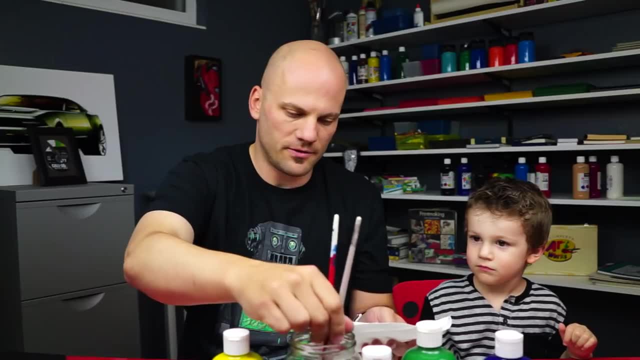 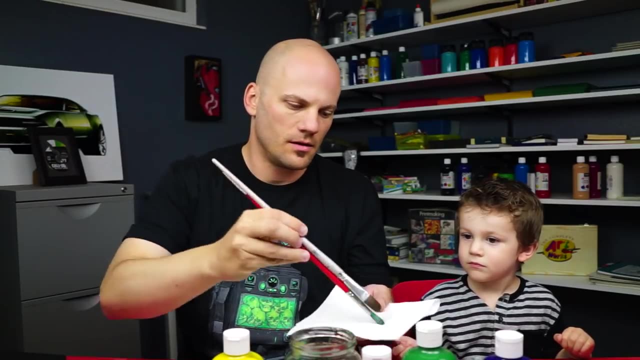 to rinse it out. Can you get the green off your paintbrush and put it in here? I'll help you. It's kind of hard to reach, huh. And then we got our paper towel. We'll dry it off, All right, Okay. okay, here you go. Here's your paintbrush back. Okay, now we're going to do a. 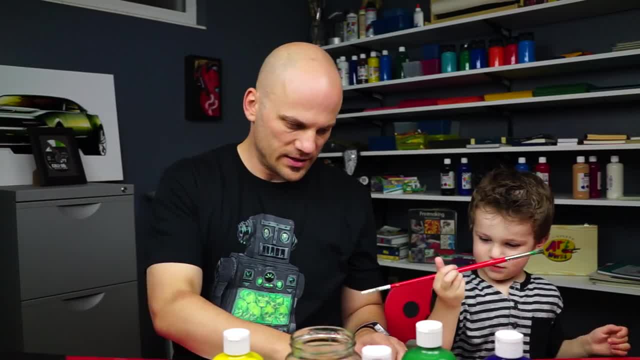 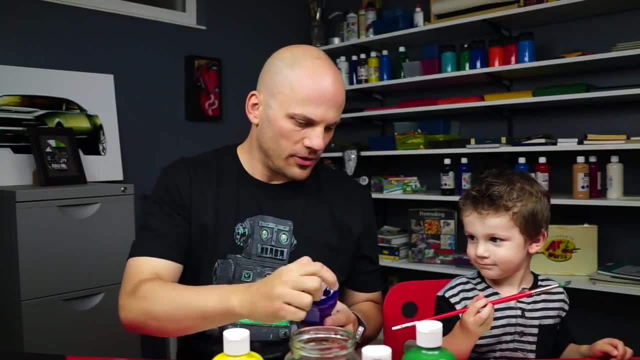 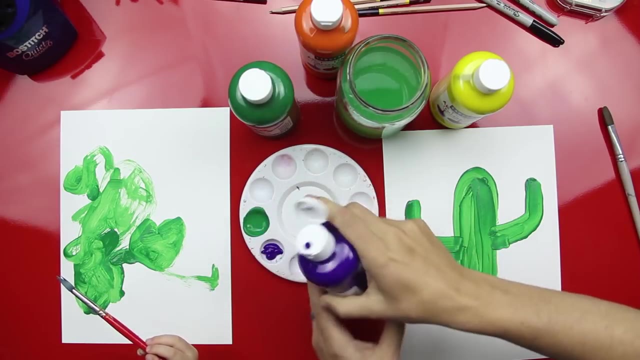 different color. All right, you ready for this? We're going to do purple and we're going to do little flowers, Little flowers on our cactus, okay, So watch Dad, Watch this. You get a little purple on our. 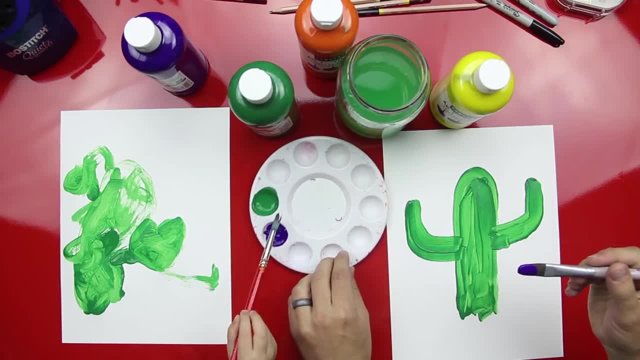 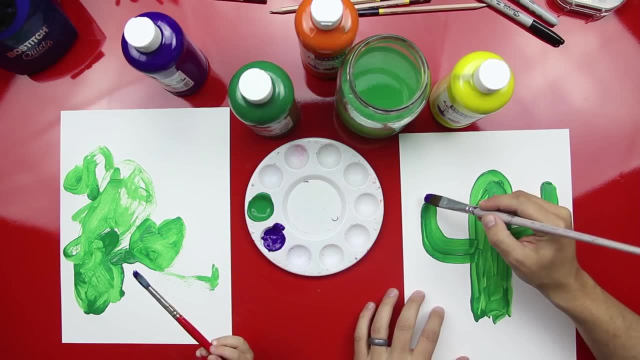 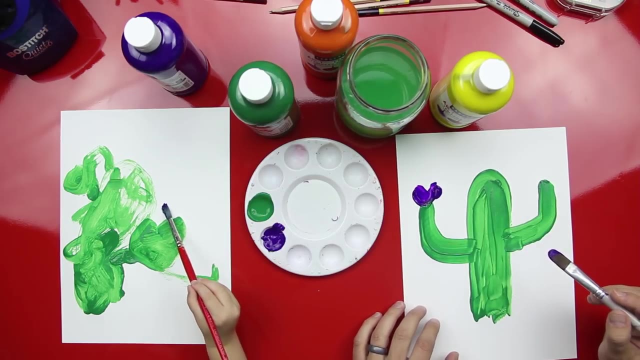 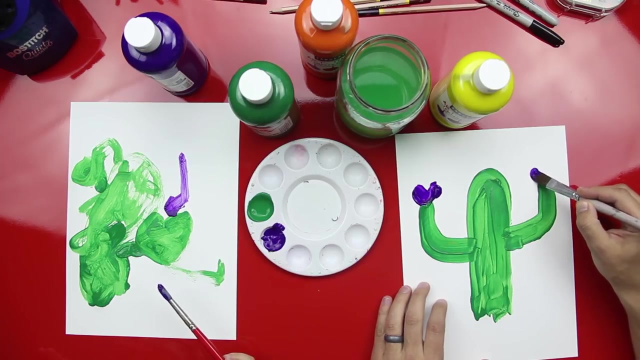 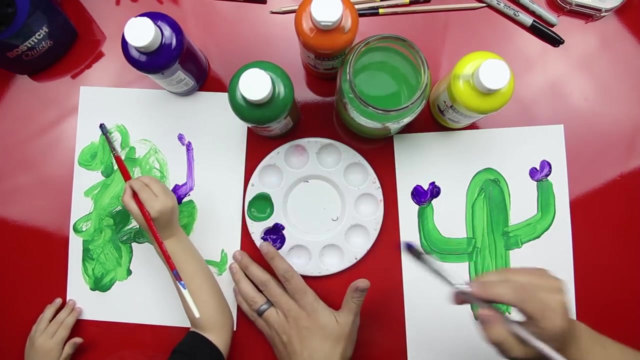 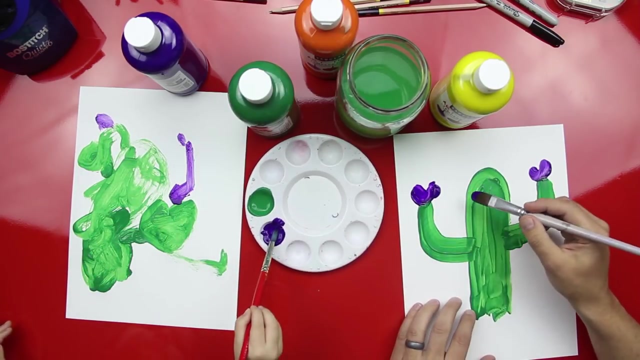 paintbrush. Get some on there, Get a little more. Yep, good job. Okay, all right. now we're going to do a little- just a little U- on top, Down and then up. Yeah, okay, stop. Oh, there you go. Good job, Kate. And then we're going to do another one over here, Down and then up. Little U, Can you do it on this side over here? Do a little one right there. Good job, buddy, Good job. Let's do one more. And we're going to do it on the side, right here, Down and then up. 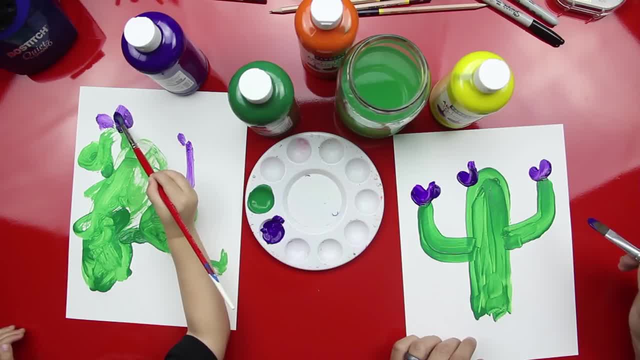 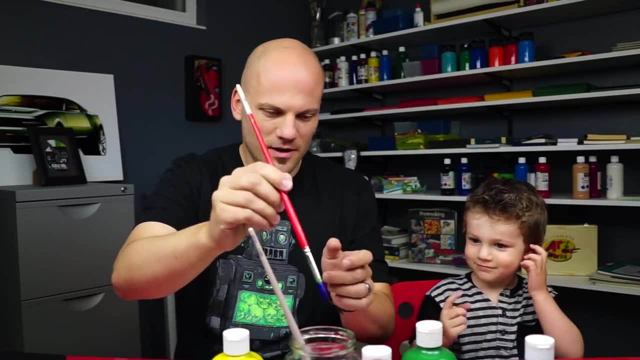 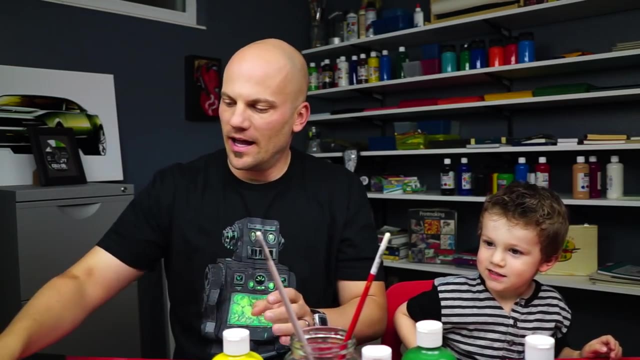 Down and then up. Yes, good job, Austin. how old are you? again? Two, Yes, Austin's two. so we're trying to keep the steps very simple and I think it's good to give them a little direction, but then let them do it. 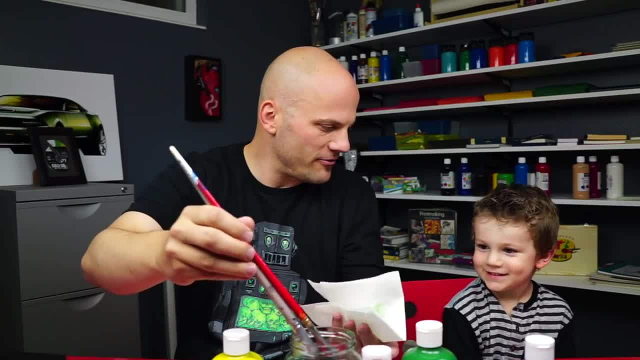 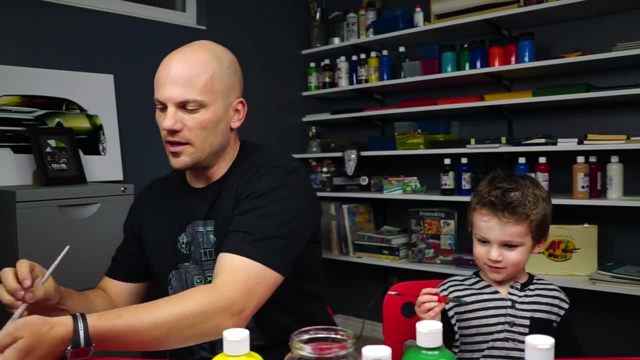 Don't want to do it for them, Just let them have fun. huh, You having fun? Yeah, Good, All right, want your paintbrush back? Yeah, Okay, we got the purple off. Now we're going to do a little yellow, and it's just going to be a little bit, and we're just going to make a oops. 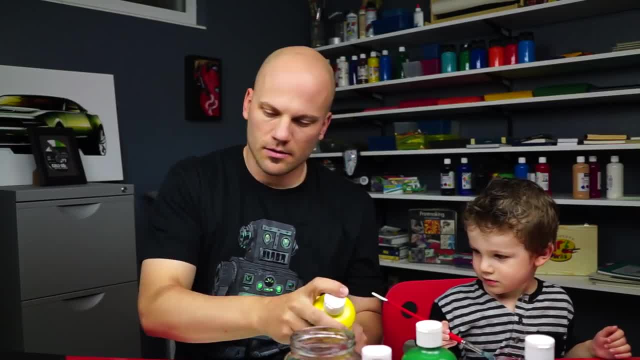 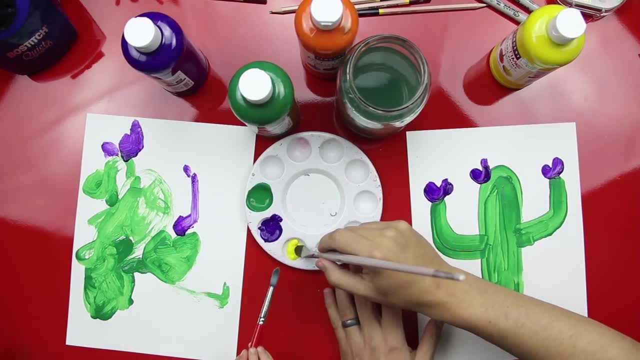 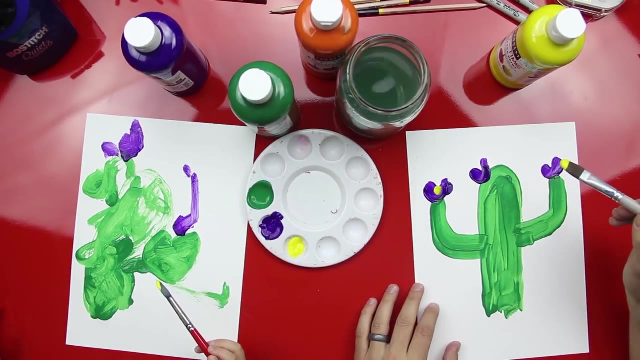 Kind of splash there, squirt it out. Okay, we're going to do. get a little yellow on your paintbrush. Okay, just a little bit. There you go, Good job. Okay, watch dad, You're going to do dot. Can you do a dot? 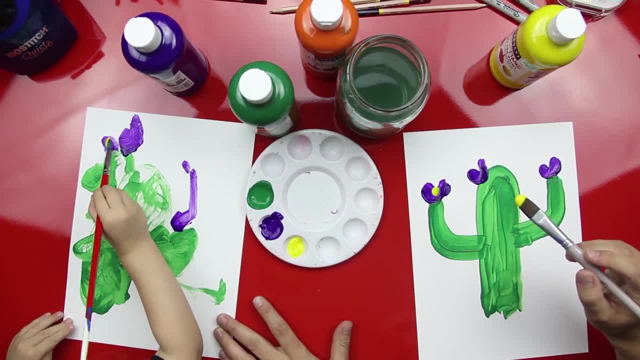 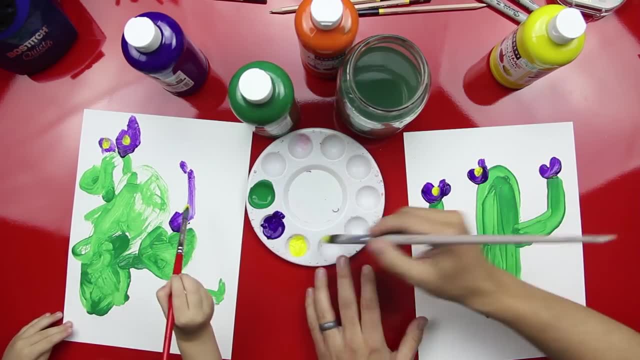 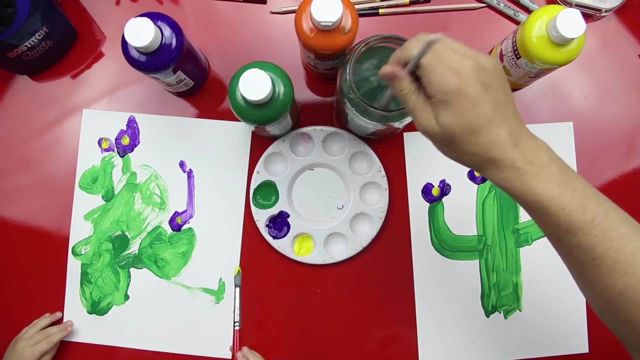 Yeah, Do a dot on the purple Dot, Good job, Get a little more, get a little more yellow, Good. And then another dot, Yep Dot, And another dot. Yeah, That's the inside of the inside of the flower. Okay, let's get the yellow off. and then we're going to do the orange. 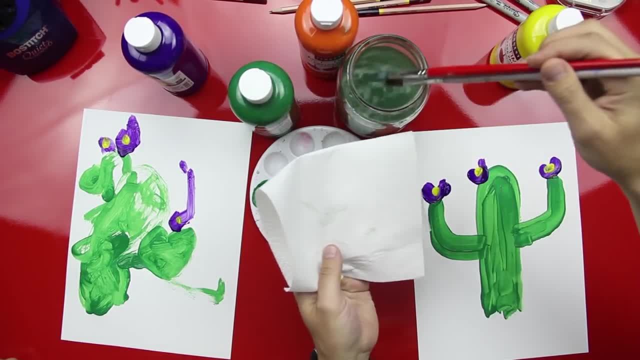 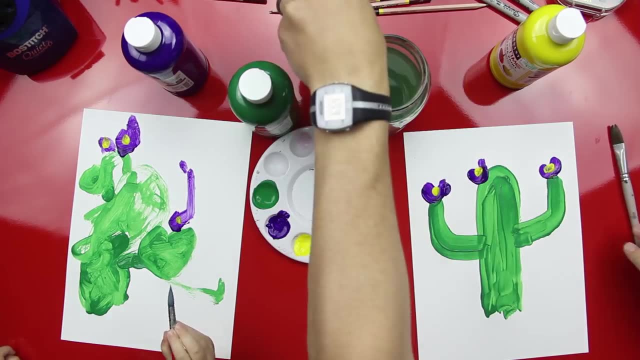 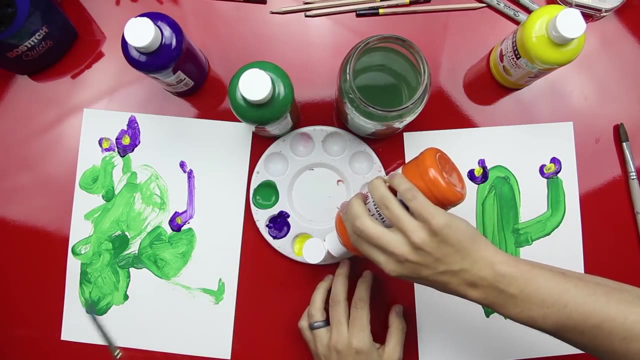 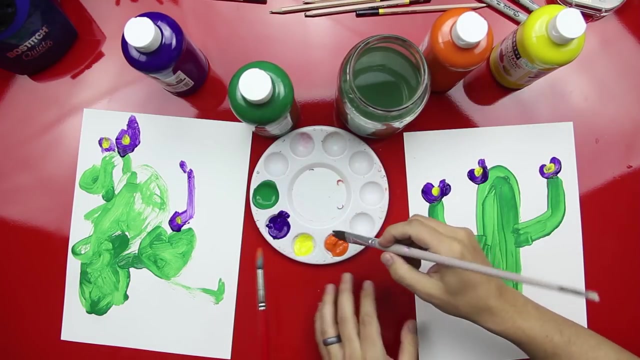 Orange, Orange. Here's your paintbrush. You ready for the orange? Yeah, What are we going to use the orange for? Do you know? Rocks, Rocks, Desert, Desert, Desert, All right, Okay, we're going to do a little orange and we're going to make big ovals down here. Watch this, Okay. watch dad first. 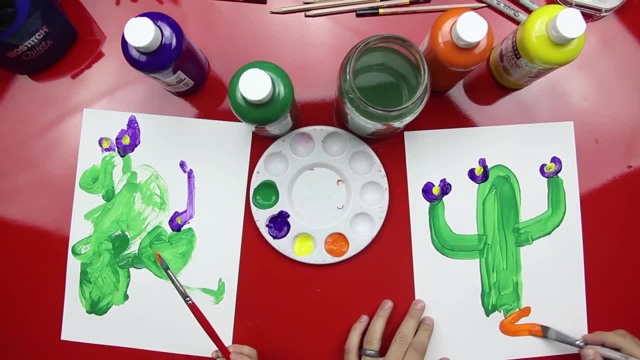 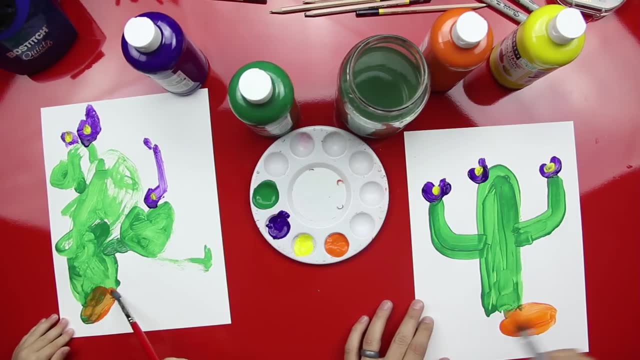 Okay, we're going to make a big oval down here. Watch down at the bottom, make a big oval. Can you do a big oval down there? Yeah, Do a big, big, big. Yes, good job, And you're kind of mixing it with the green. huh, Here, let me get the. we'll do a rinse it off. 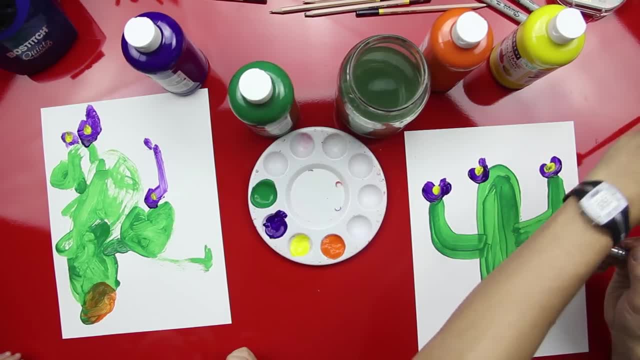 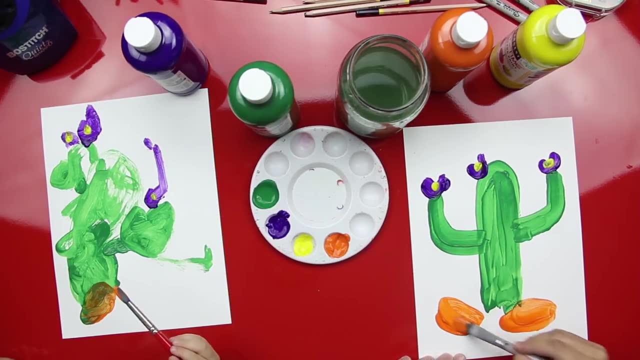 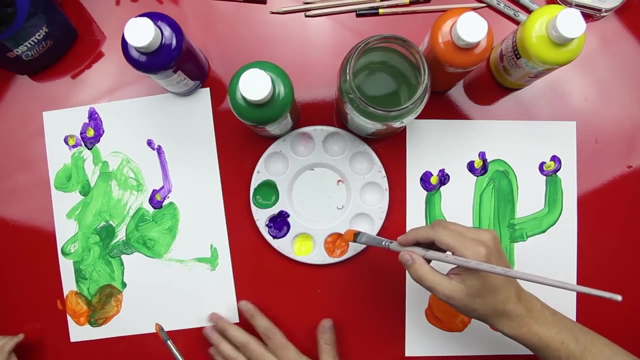 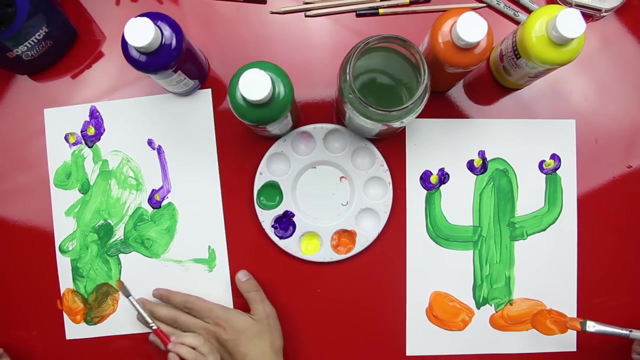 Again, get the green off. Okay, get some more orange. More orange, Okay. and then we're going to do a big oval over here. Good job. Okay, get a little more orange, That's okay, we'll wipe it off, It's okay. Okay, get a little more orange. Okay, do a big oval over here, Right over here, Right here.